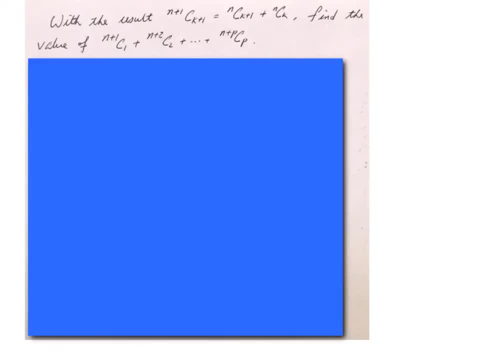 Right. this is another problem about binomial theorem. In this case we use this result: okay, n plus 1 c k plus 1 equals n c k plus 1 plus n c k. You can prove this by simplifying the right-hand side by using the definitions for ACRL: Right, if we have this result and 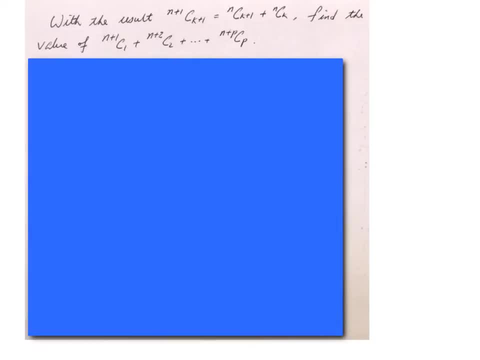 then we are asked to find the value of n plus 1, c 1 plus n plus 2, c 2, okay, up to the term n plus p, c, p. Now if you first look at the look at this series, you can think whether we can say group these two terms together. 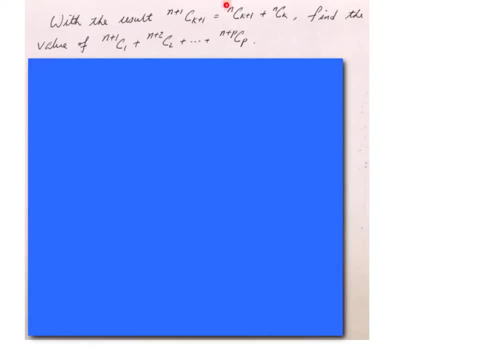 into one term like this and it becomes one term And then maybe okay, after grouping these terms together, the results can be grouped with other terms like that. But if you look carefully you will see that we cannot apply the given results directly, say, for these two terms. Because if you look 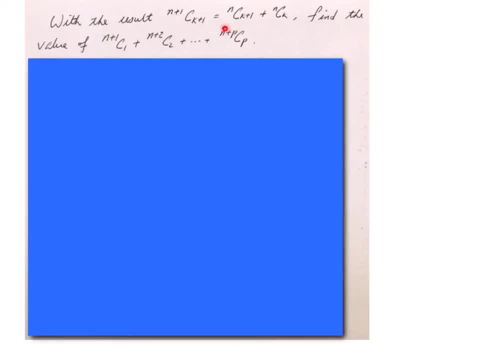 at the right-hand side. okay, of these two terms here they are having the same n here- One is n c k plus 1 n c k. But in this case, if you look at these two terms, this is n. 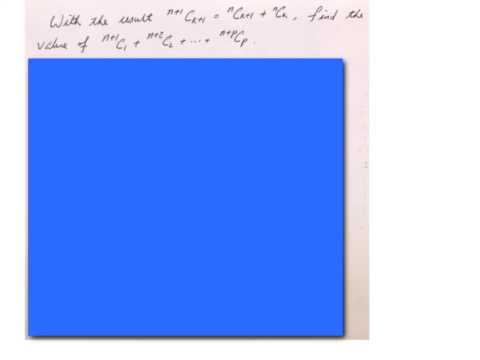 plus 1.. This is m plus 2.. And then for the coming terms, they are all different. okay, The next term afterwards should be m plus 3, and it's C3.. Therefore, we cannot apply directly this result. 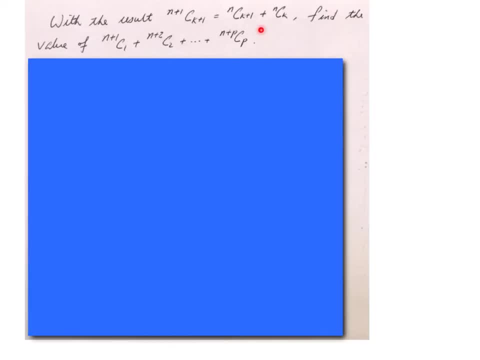 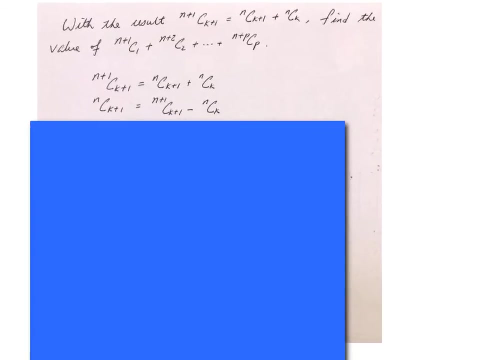 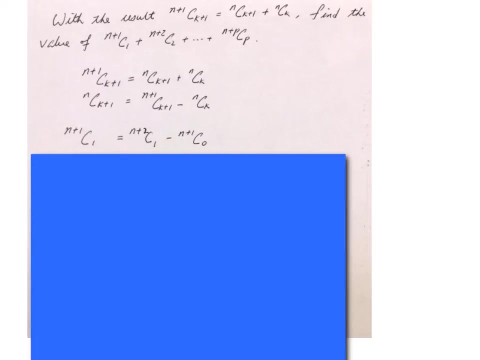 And then how can we simplify this one? If we don't know exactly how many number of terms are there In this case, we may consider by rearranging the terms. Rearranging the terms And then we create a difference. And then if we make use of this result, say, we rewrite m plus 1, C1 by applying this result. 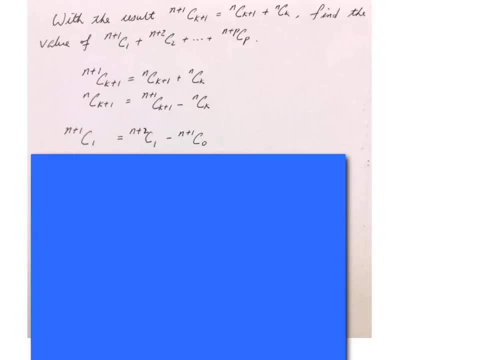 then you can compare. okay the terms: Here is n, This is m plus 1.. Therefore, if we look at the pattern, if this is n, here this is n plus 1.. Therefore, if this is n plus 1, then this is n plus 2.. 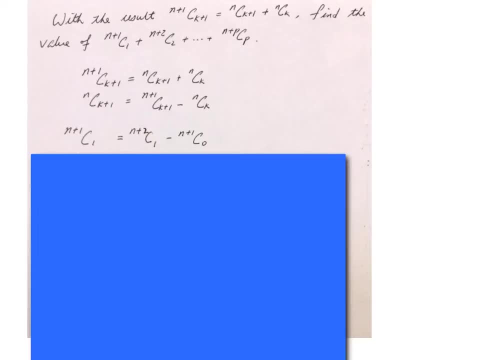 If this is k plus 1, this is k plus 1.. Therefore, for this one, it is 1.. This part is 1.. And then minus. okay, if this is n, this part is n. Therefore, for this one, it is n plus 1.. For this term, it is also n plus 1.. 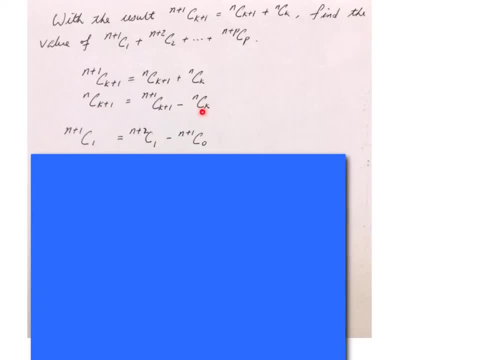 And then we look at the index, here k plus 1.. Therefore, this term, it should be k. Therefore, for this one, it is 1 here. Therefore this is 0.. And then we try to do the same things for the remaining terms. 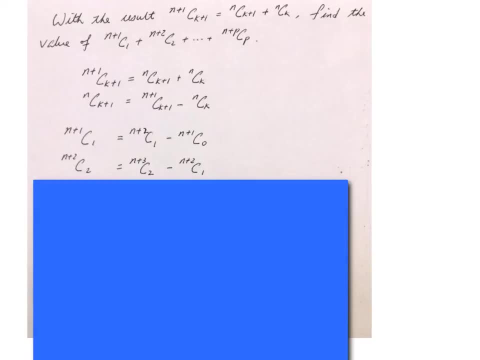 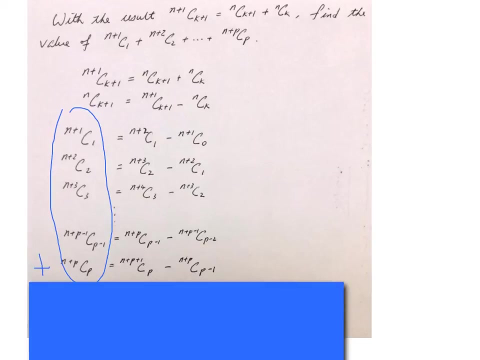 Like m plus 2 C2, will be rewritten as m plus 3 C2 minus m plus 2 C1.. And then we continue After this term And then, in this case, if we add the terms vertically, okay, this is the required sum.